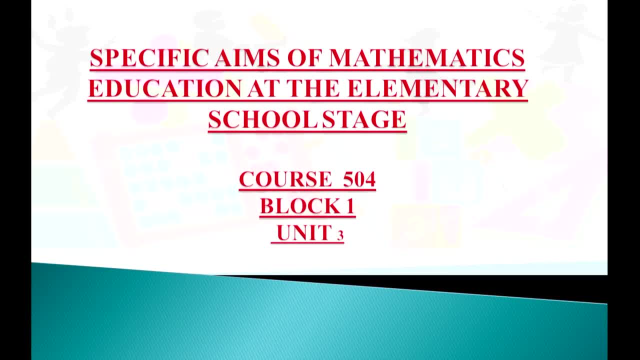 Hello learners. I am Shivani Bali teacher educator. Today we are going to learn specific aims of education at the elementary school stage. This topic is from course 504, block 1, unit 3.. Before explaining the specific aims of elementary education, let me give 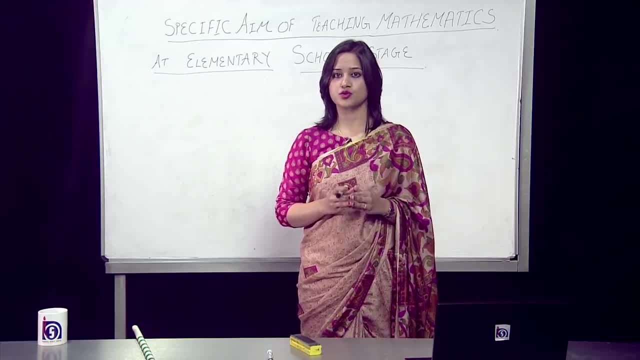 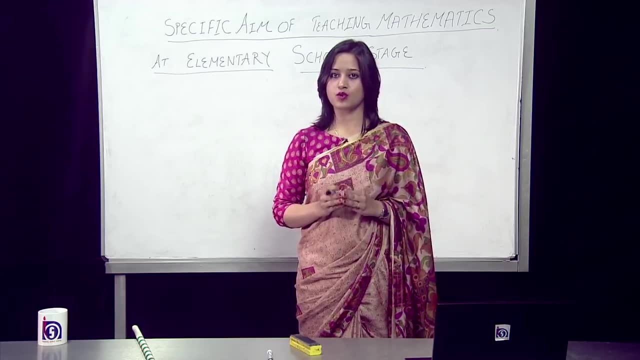 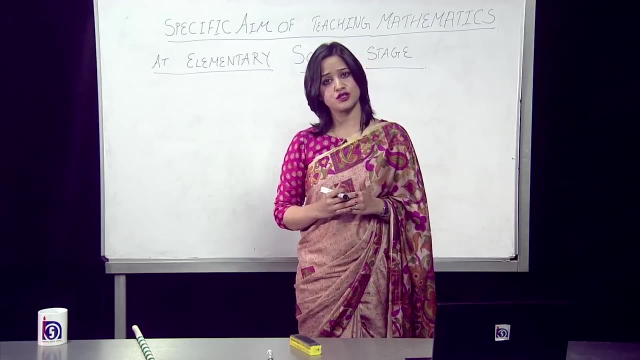 you the brief history. In India there is uniform education structure which we call 10 plus 2 plus 3 pattern. This pattern was adopted in post-independent India on recommendation of education commission. So, based on the reports of education commission, government of India. 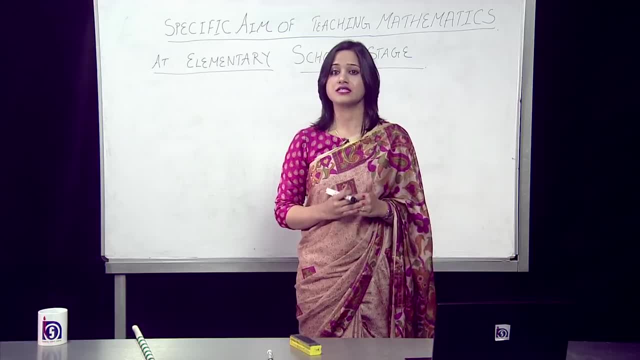 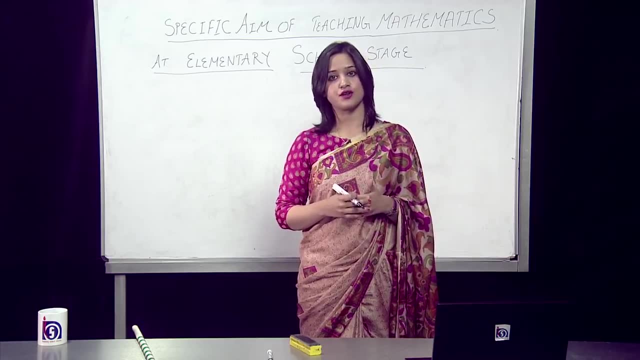 first announced the national policy of education in 1968.. As per this policy, all school will provide compulsory education to children. In the article 21A of Indian constitution it is also mentioned that free and compulsory education would be provided to all children of age group 6 to 14 years, which form the 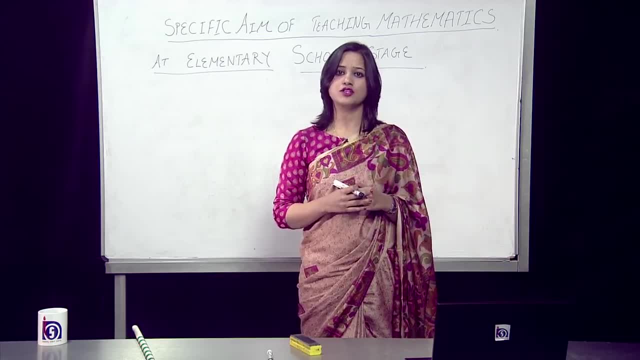 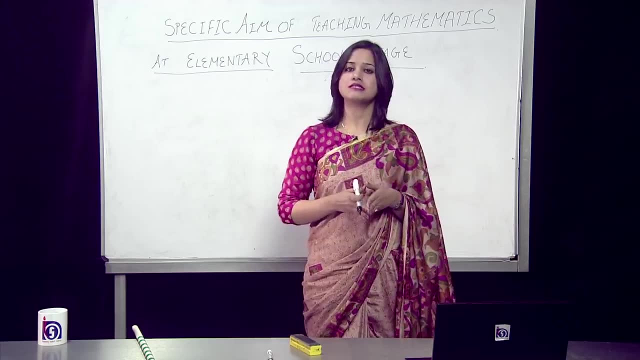 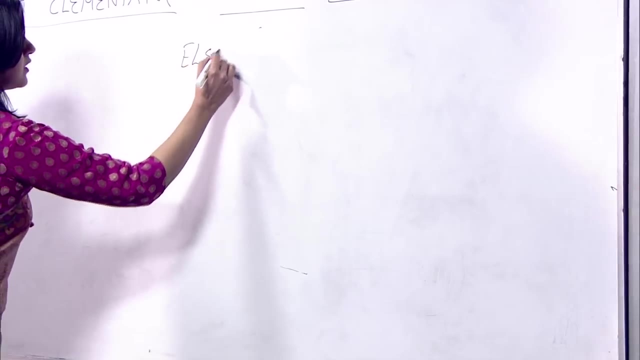 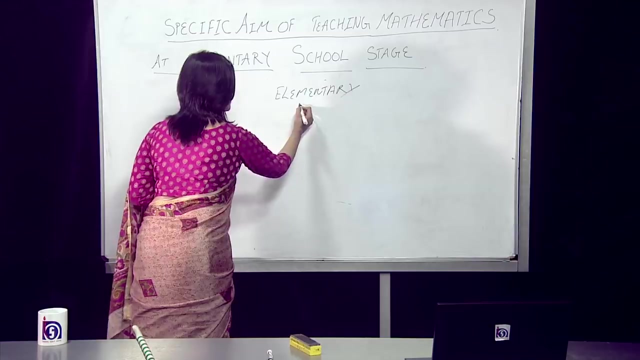 basis of Right to Education Act. Now formal education of these children of age group 6 to 14 years comes under the domain of elementary education. Now let's see the structure of elementary education. 1. Elementary education covers the children of 6 to 14 years of age group, from class 1st. 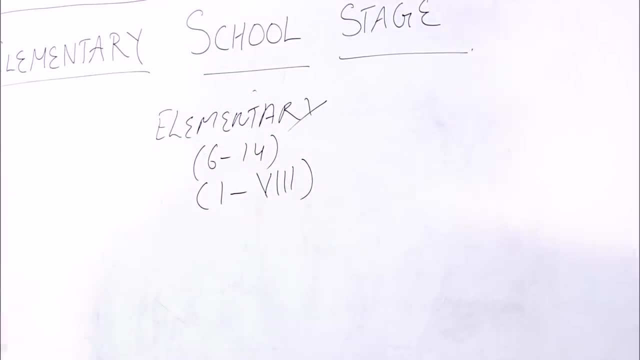 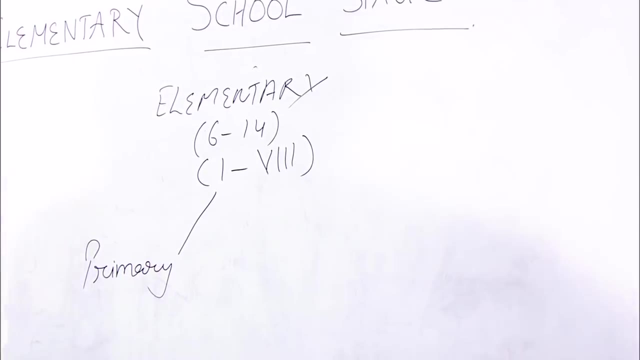 to class 8th. It is further subdivided into two levels: primary and upper primary 2. Elementary education covers the children of 6 to 14 years of age group, from class 1st to class 8th 3.. 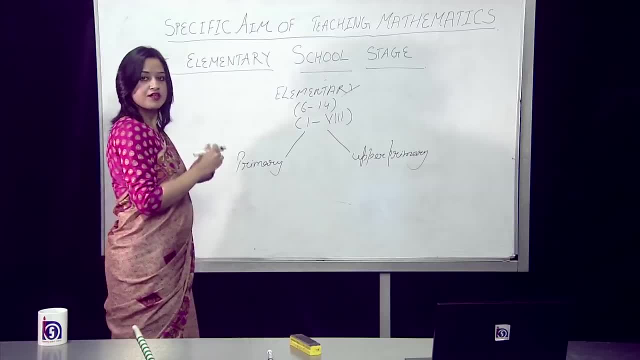 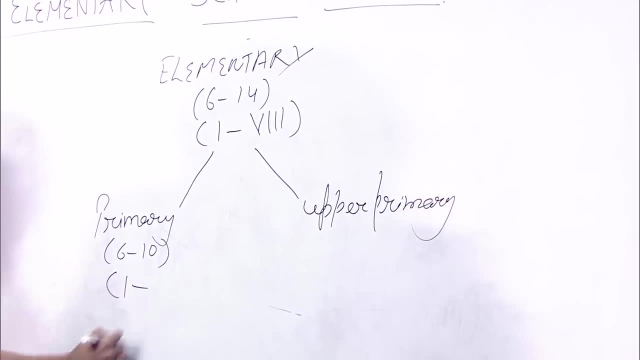 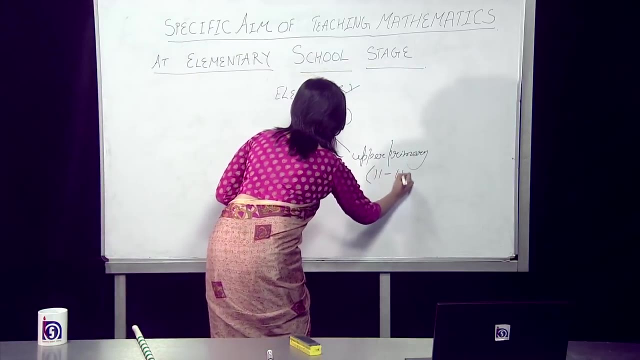 Primary level covers the children of age group 6 to 10 years, from class 1st to class 5th. 4. Upper primary covers the children of age group 11 to 14 years, from class 6th to class 8th. 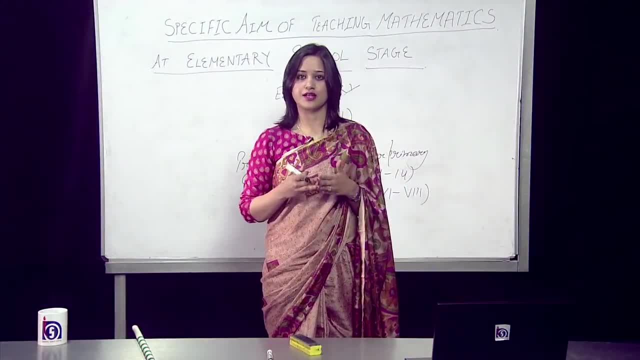 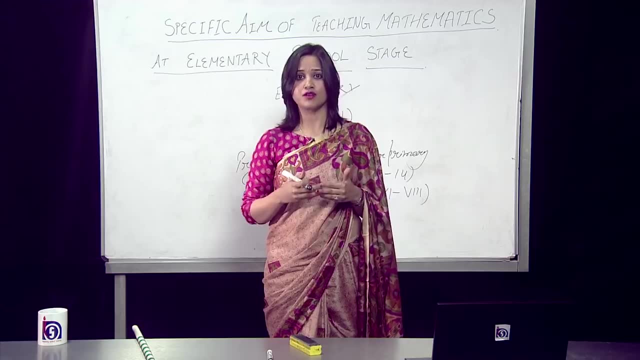 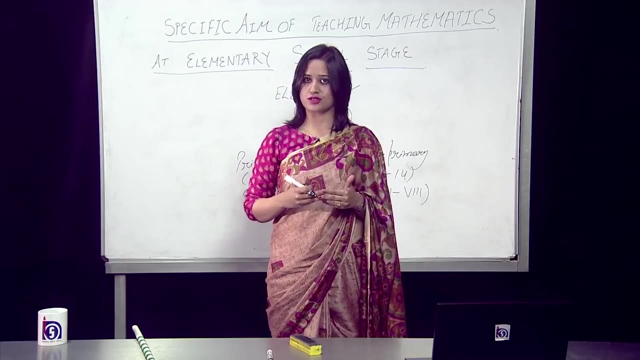 Now, what are the goals of mathematics education at elementary level? As per the guidelines of National Curriculum Framework 2005,, which is one of the important framework of India, the main goal of mathematics education is to build abilities of Mathematization in students. 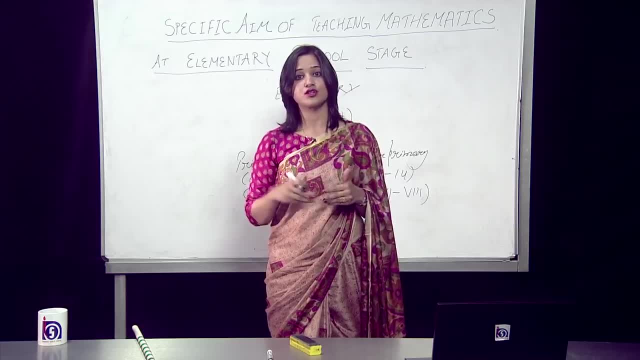 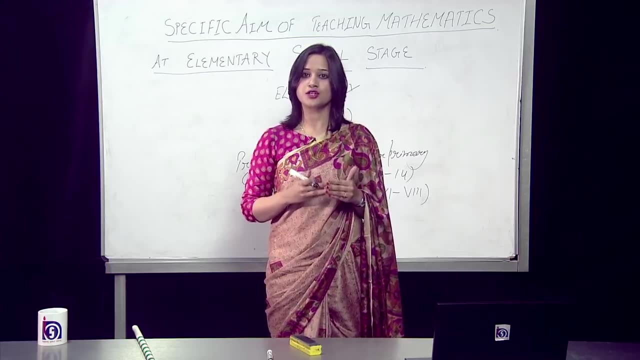 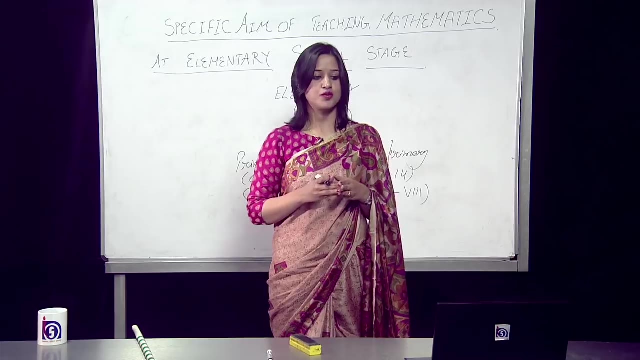 So by Mathematization we mean to bring mathematics in the thought process of a child to enable students to solve real and practical problems. Children should learn to think about any solution using the language of mathematics. Child should be able to make connections between mathematics and everyday mental activities. 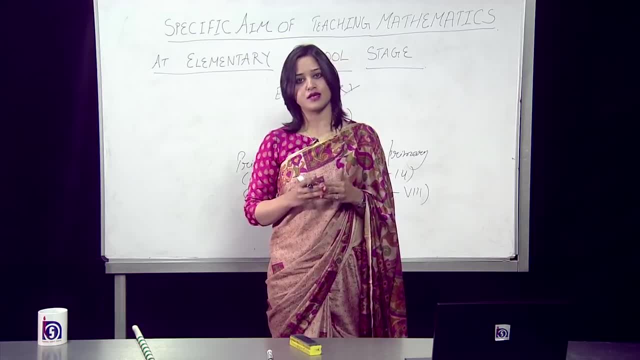 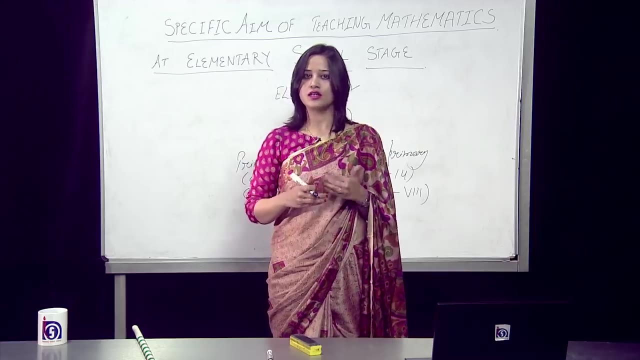 Students could appreciate the beauty of mathematics in nature and its application. There should be the development of cognitive domain, enhancement of problem solving skills, critical thinking, analyzing reasoning and decision making. So these were the goal of mathematics education. Now let's discuss the specific aims. 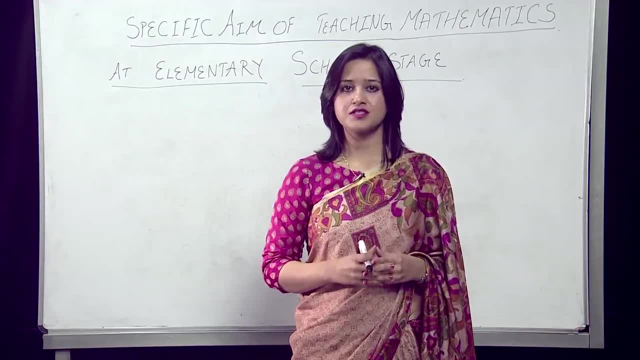 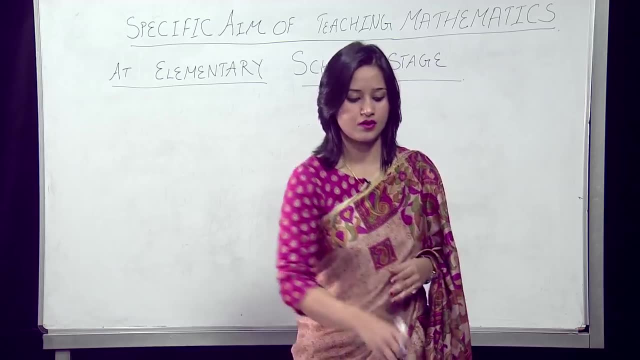 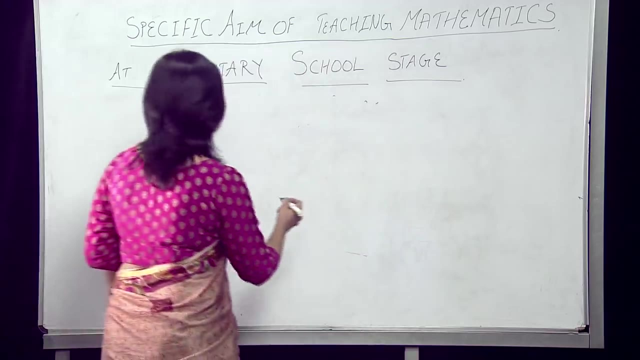 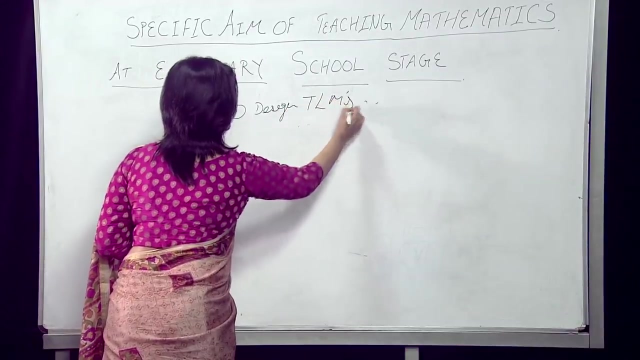 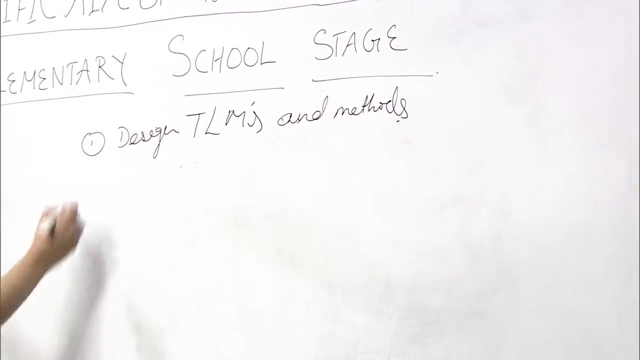 So what are the specific aims of teaching mathematics? Specific aims, Specific aims of mathematics education, are the instructional objectives of particular topic or lesson. Specific aims helps to: first, design teaching learning materials and methods. Second, develop the knowledge of mathematics. Second, develop the knowledge of mathematics. 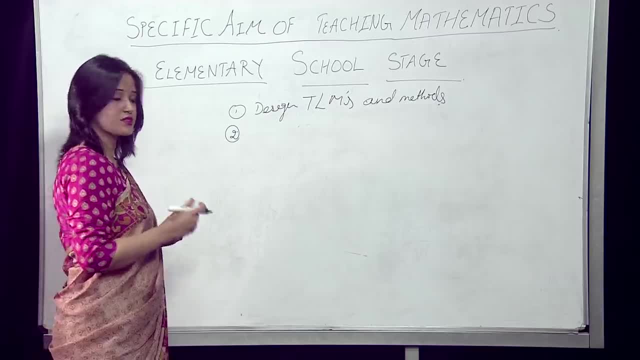 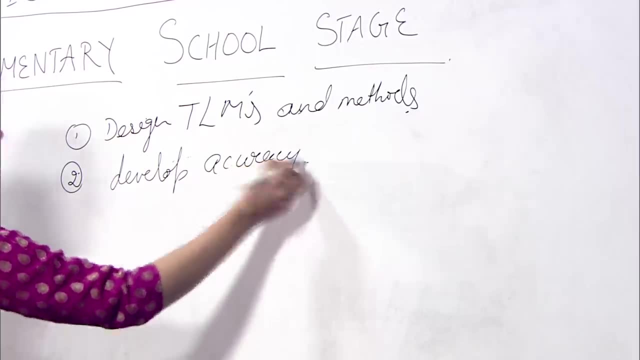 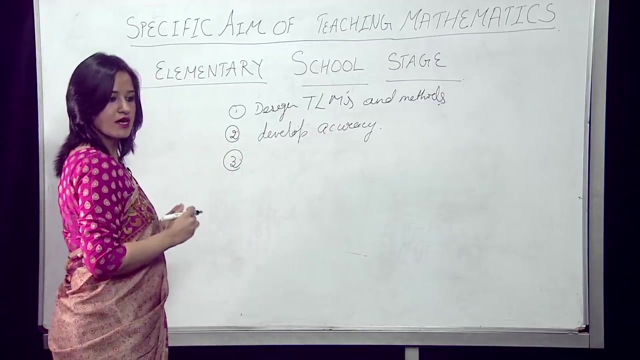 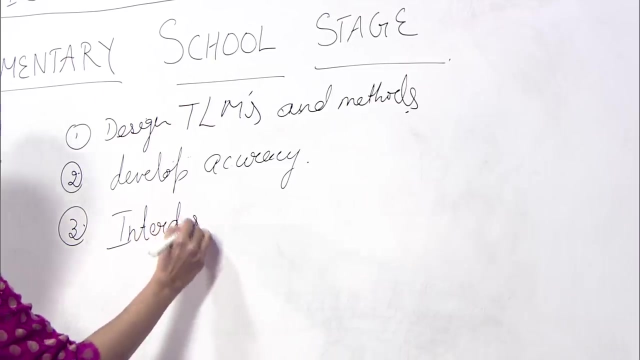 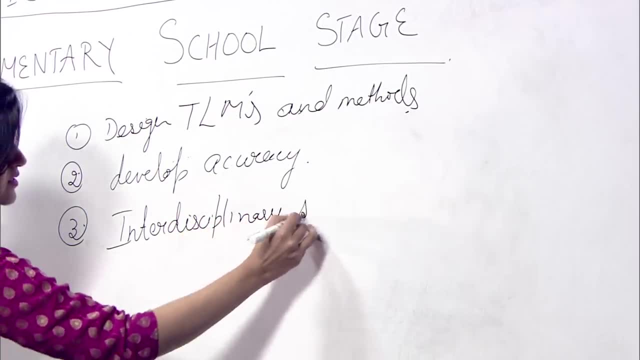 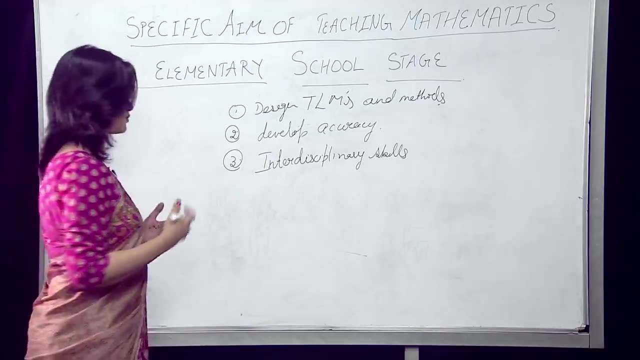 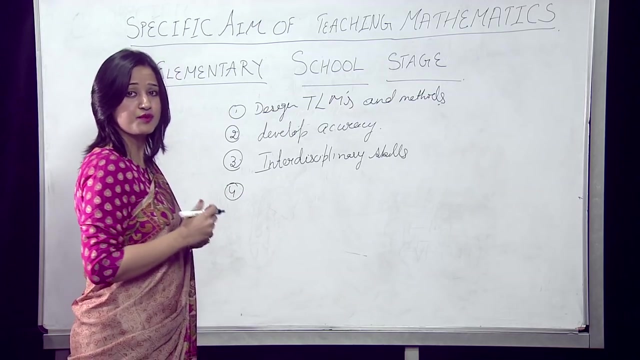 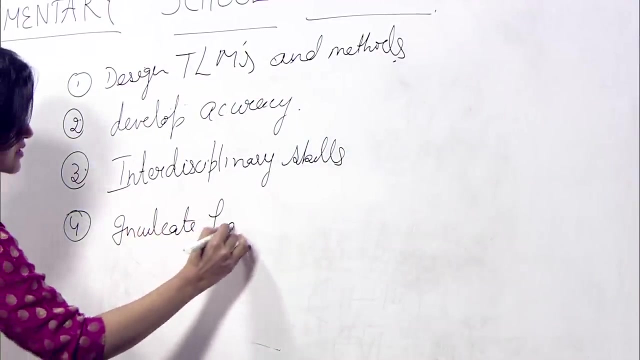 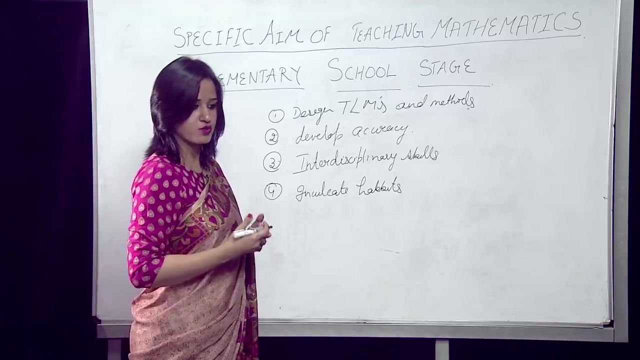 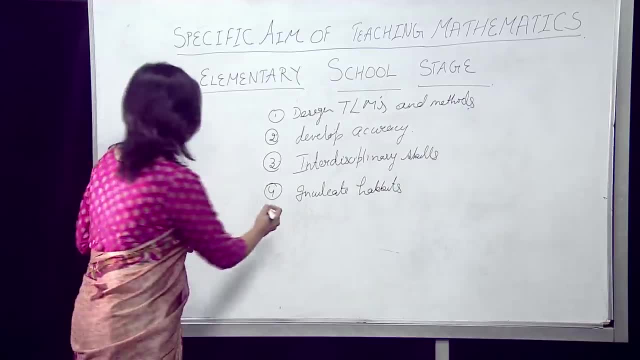 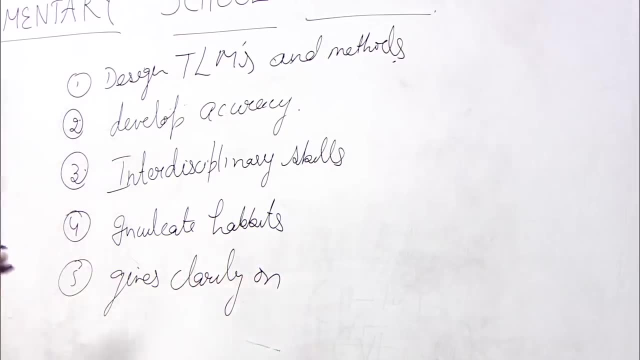 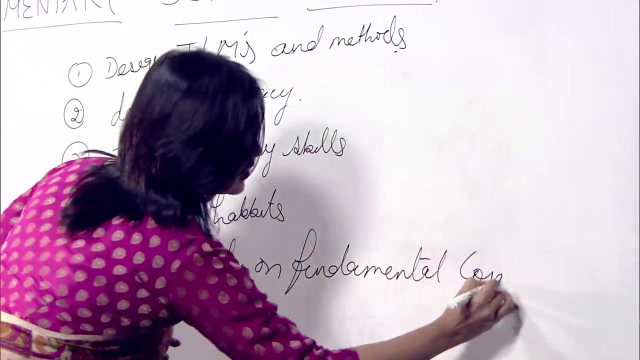 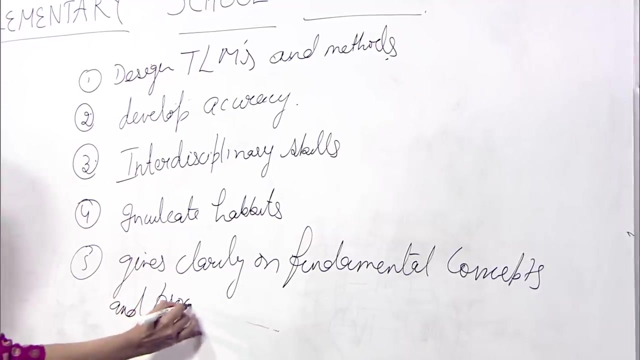 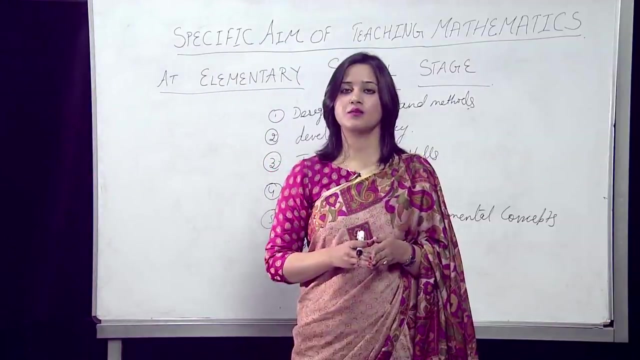 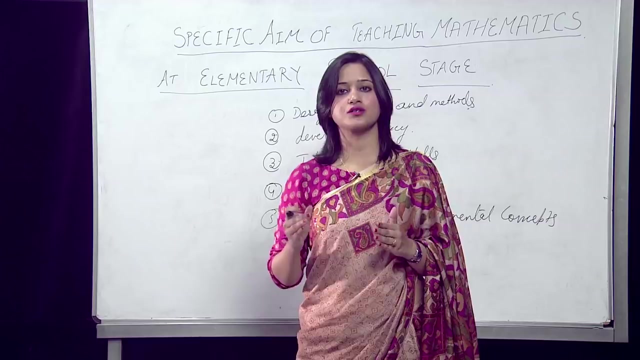 clarity on fundamental concepts and processes gives clarity on fundamental concepts and processes. So these are the specific aims of teaching mathematics. For example, if we have to write the specific aim of teaching fractions, we will write. after learning fraction, students will be able to identify numerator and denominator. Second, 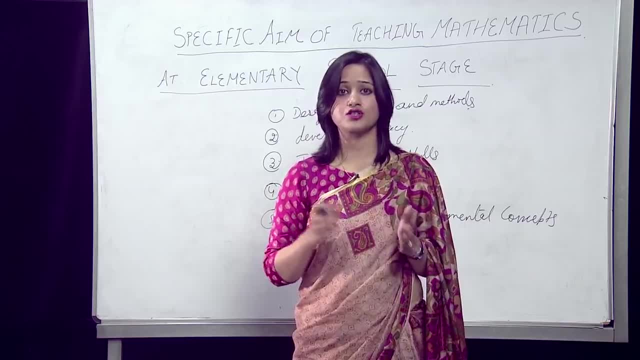 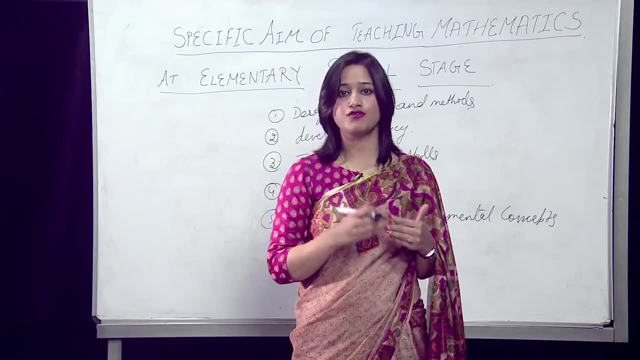 to distinguish different types of fractions, like proper fraction, improper equivalent, mixed fraction. Number three to compare and order fractions. Number four to convert improper fraction into mixed numbers to add or subtract fractions. Number five to compare and order fractions. Number six to add or subtract. 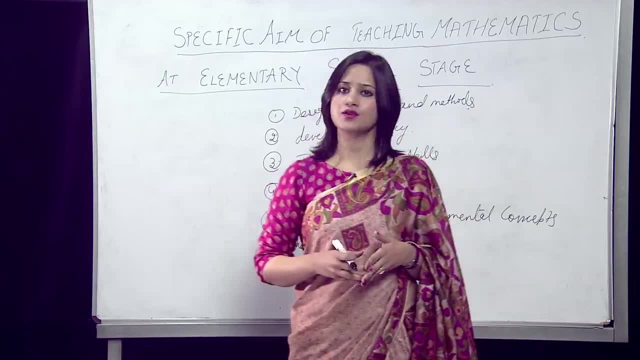 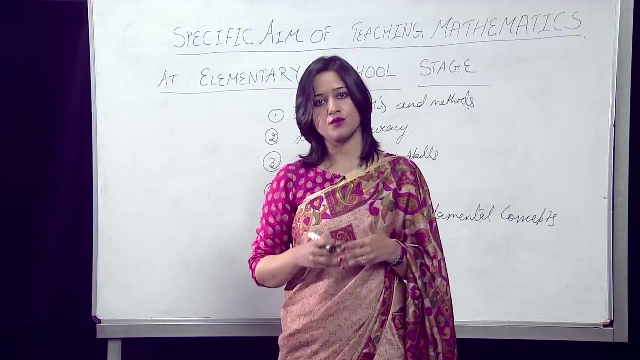 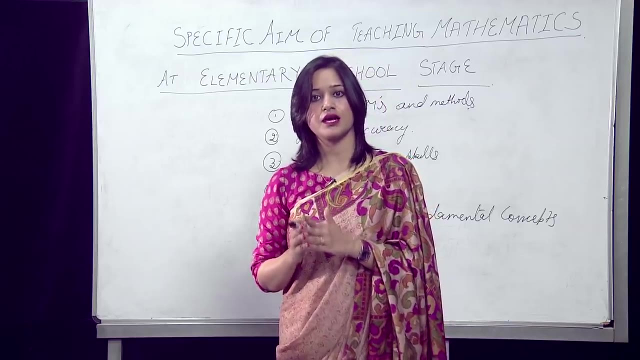 fractions with like and unlike denominators. Let's take another example where we have to find the specific aims of teaching. area of rectangle, Students will be able to define perimeter of rectangle. Number two: recognize the difference between perimeter and area. Number three, to compute the area of square if the length is given. 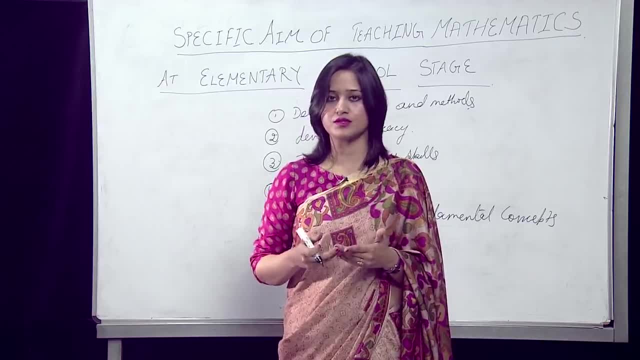 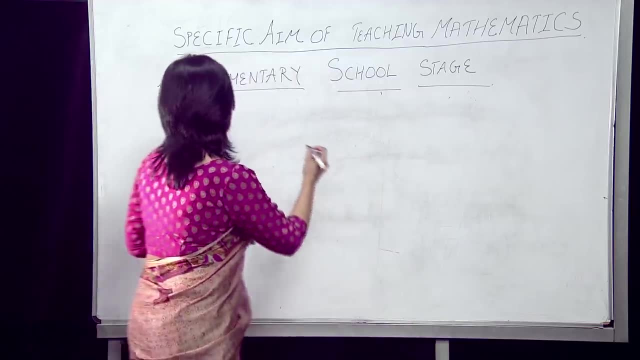 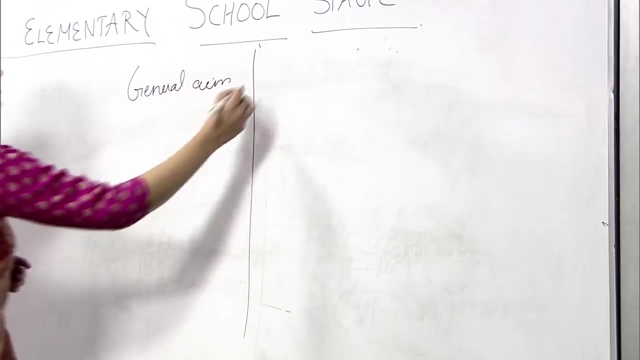 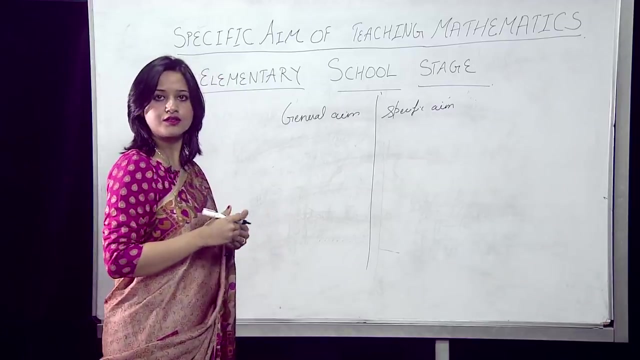 And next to apply the concept on real-life problems. Now we need to know how different are general aim from specific aims. General aims- These are the general aims of teaching mathematics, And whereas specific aims are content specific. Let's now find out other. 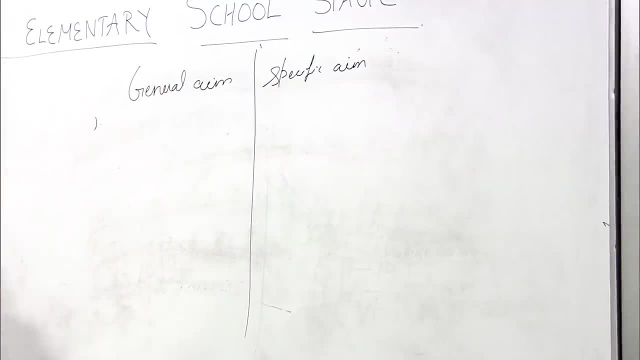 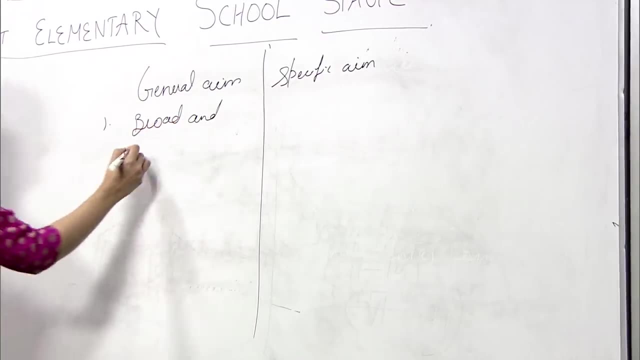 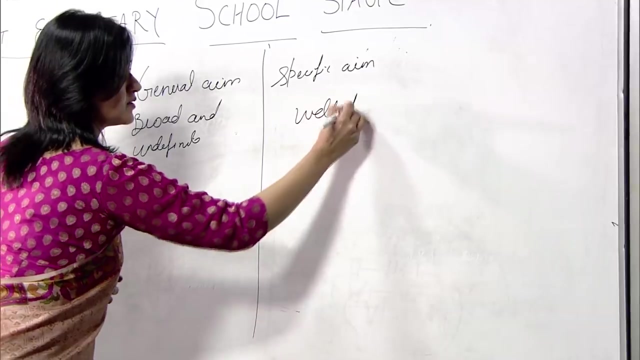 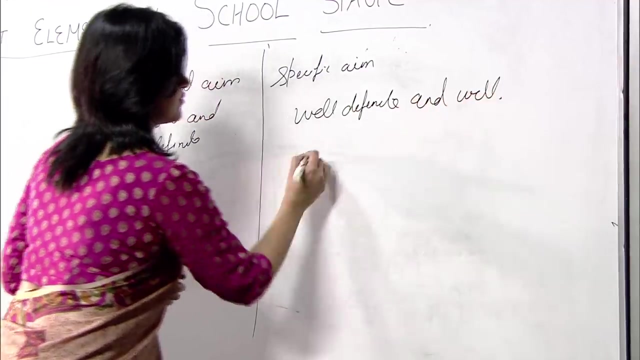 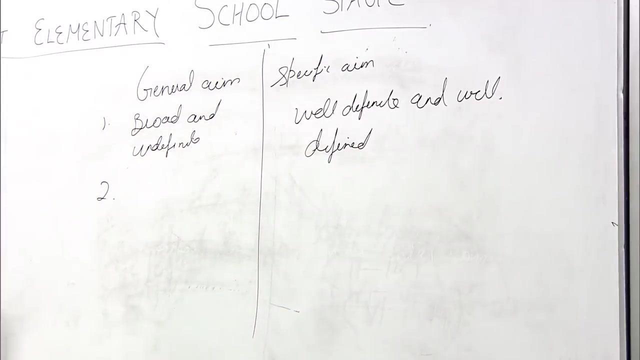 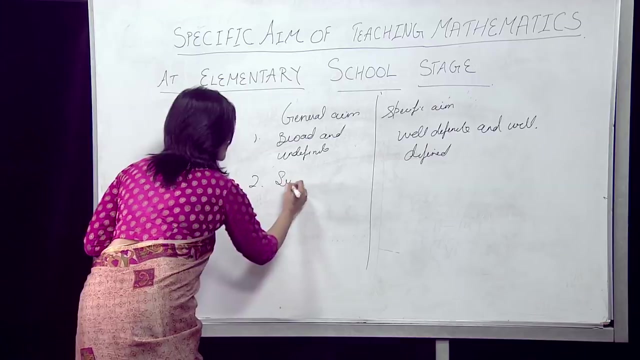 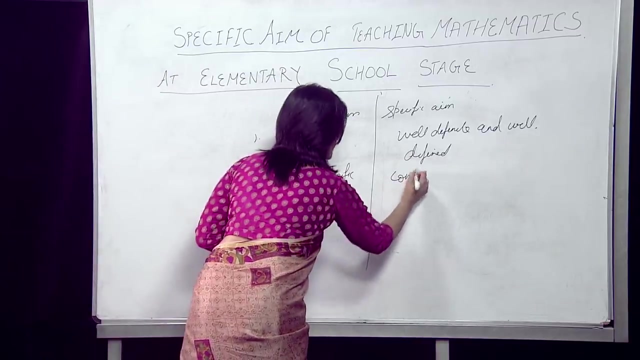 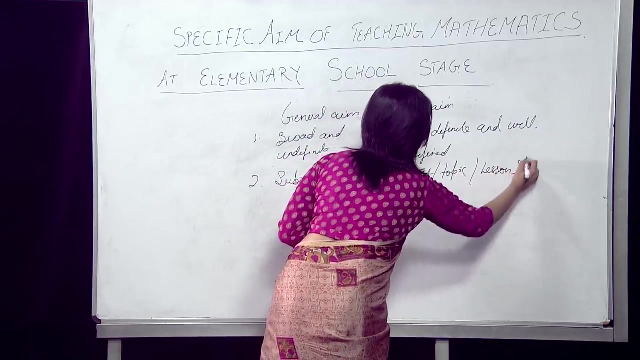 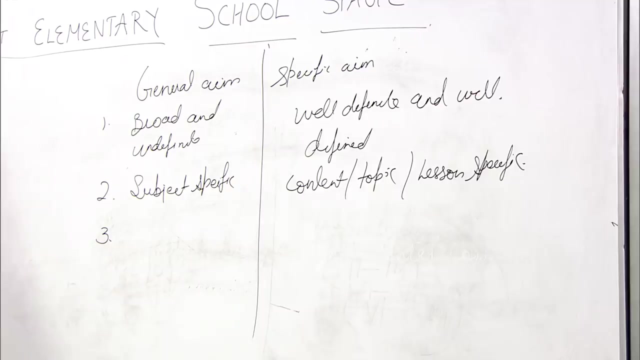 differences also. First, general aims are broad and indefinite, Whereas specific aims are well-definite and well-defined. Second, general aims are subject specific, Whereas specific aims are content specific. These are subject specific And specific aims are content or topic or lesson specific. 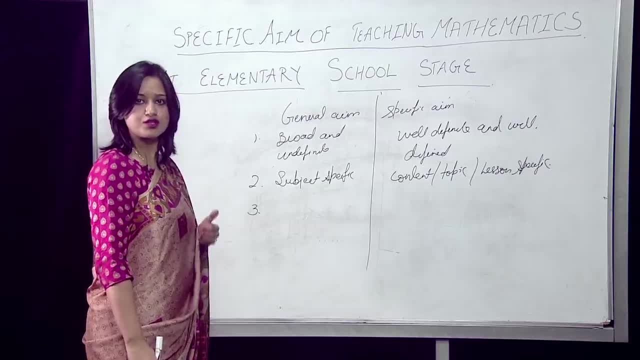 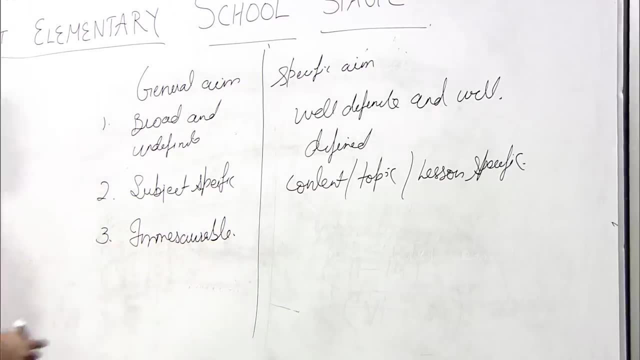 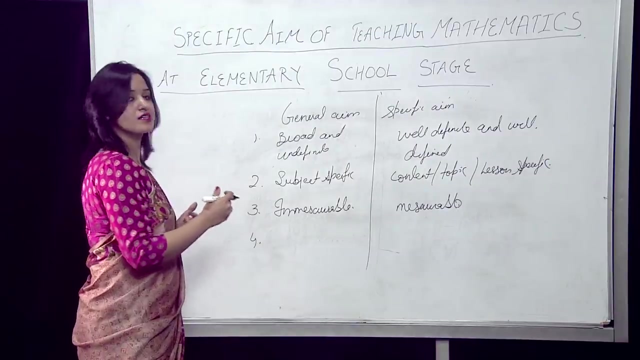 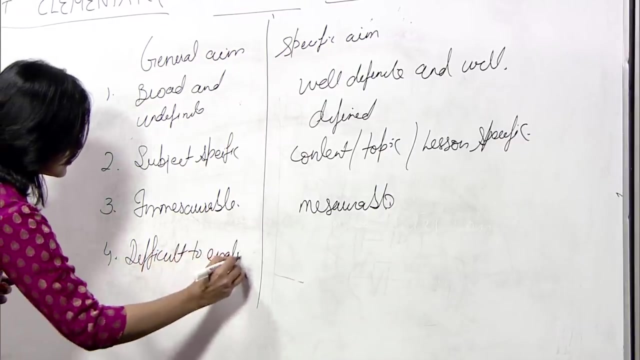 General aims are immeasurable, Whereas specific aims are measurable. They are immeasurable, Whereas specific aims are measurable. Number four: general aims are difficult to evaluate, Whereas specific aims are easy to evaluate. And specific aims are easy to evaluate. 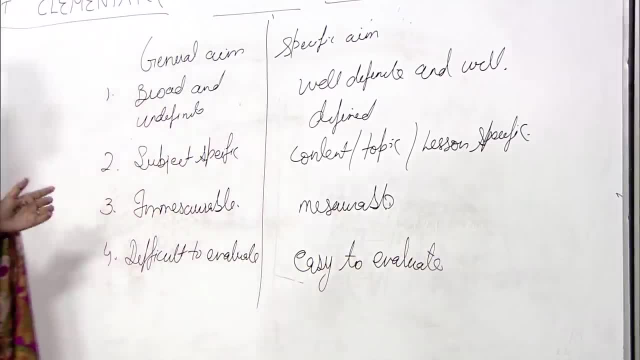 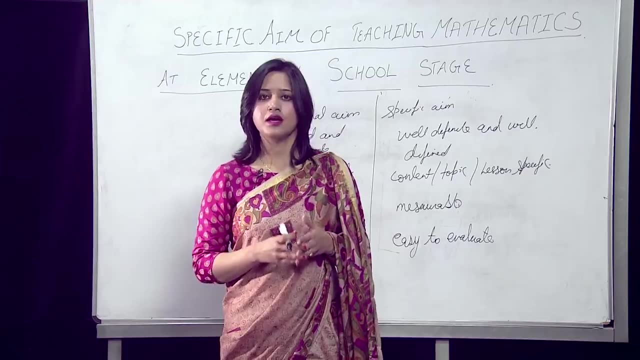 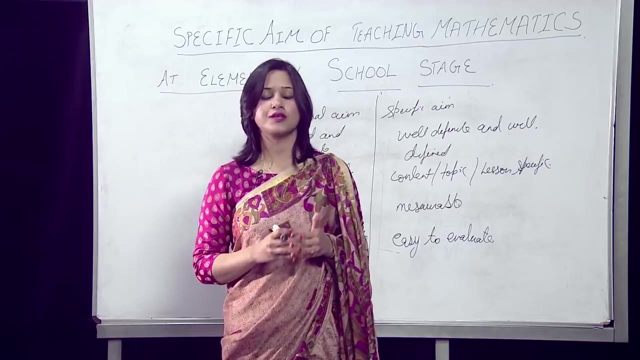 Consideration of experiences and experiences of other students is vital to support national thinking. So these are the differences between general aim and specific aims. Now let's sum up what all we have learnt. Elementary education consists of two levels: primary and upper primary. Second, the main goal of mathematics education at an elementary 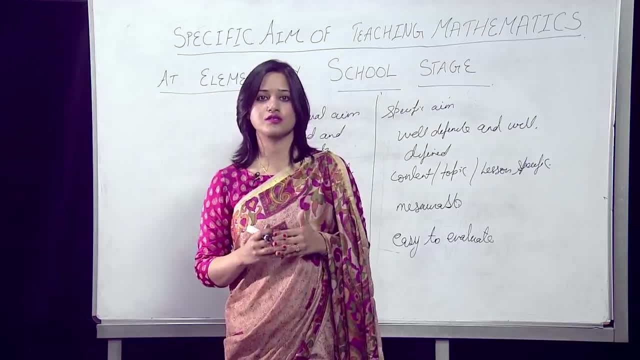 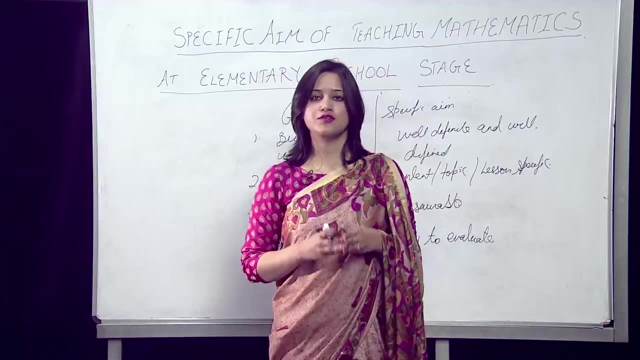 level is to mathematize children's thought process. Specific aims are instructional objectives of any topic or lesson. matter of children's thought process. Specific aims are instructional objectives of any topic or lesson. Specific aims of teaching mathematics is to develop disciplinary values, accuracy, design. 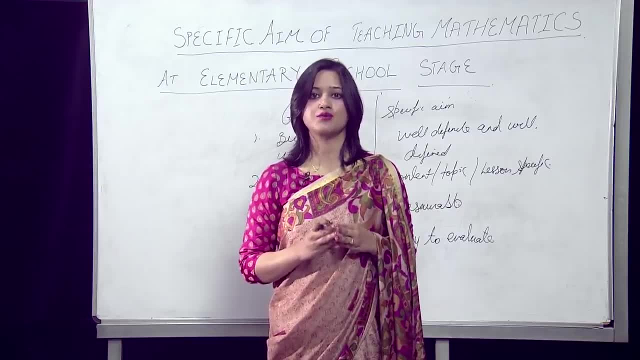 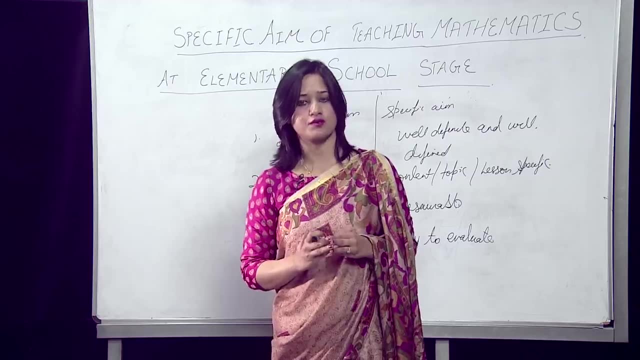 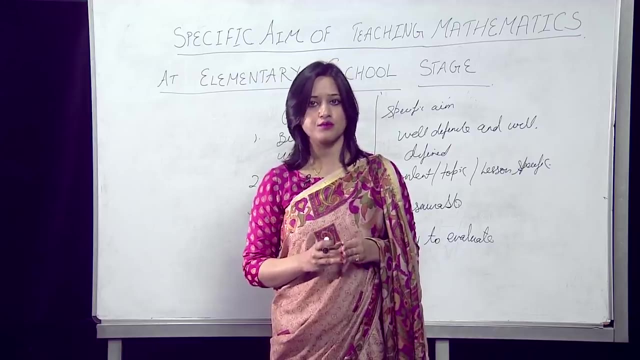 suitable methods, teaching learning materials and procedures. Specific aims are different from general aims, So this was all about specific aims of teaching mathematics. Dear learners, now let me give you a practice task. You can practice writing specific aims of teaching prime numbers or area of triangle. 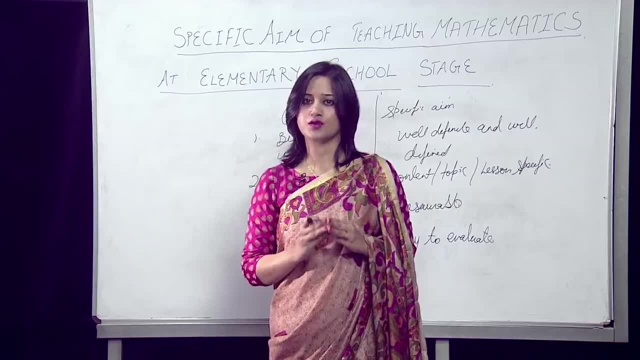 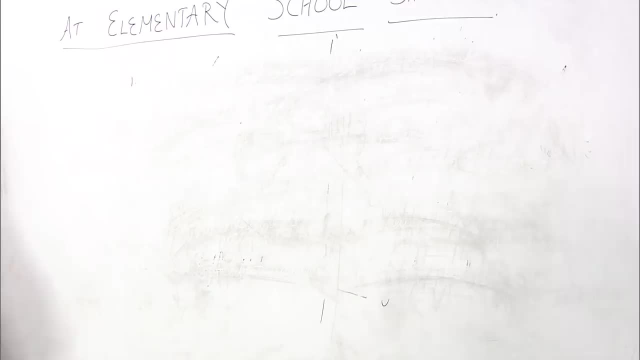 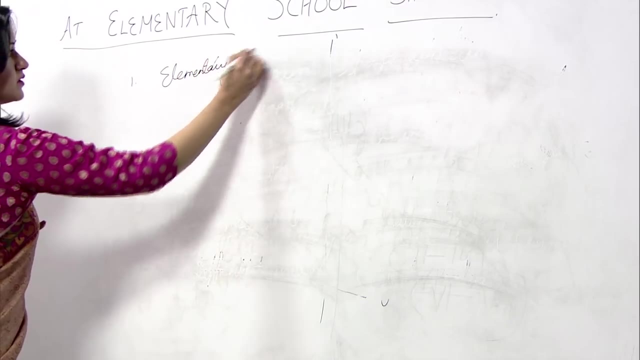 All you need to do is to write instructional objectives of teaching these concepts. So let's sum up what all we have learnt. First, we learnt about elementary education structure. in India, Elementary education is divided into two parts. First is primary and other is upper primary. 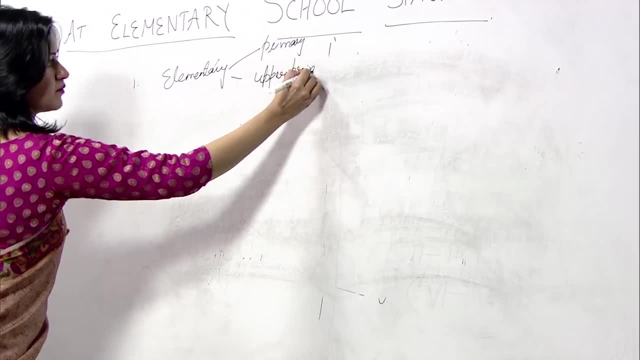 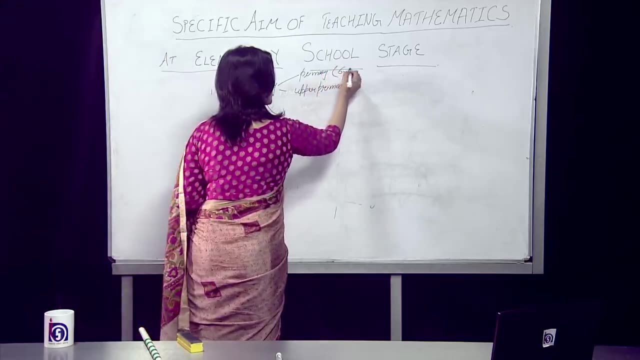 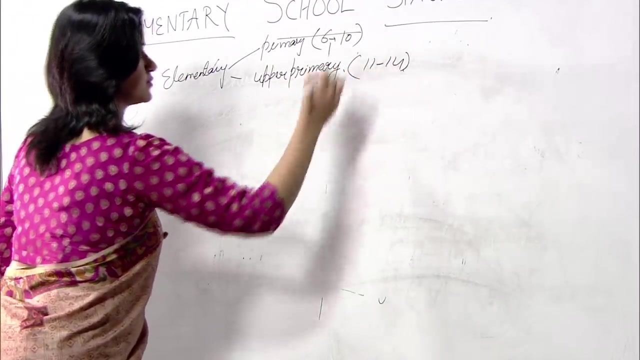 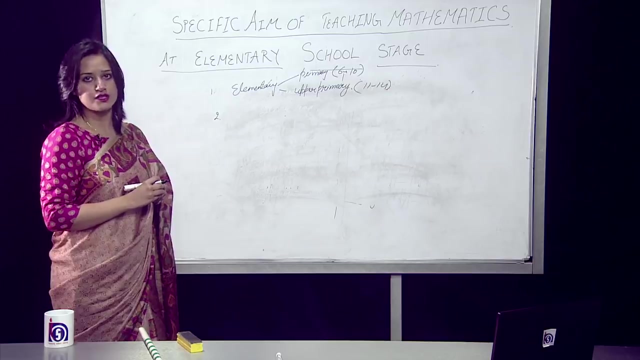 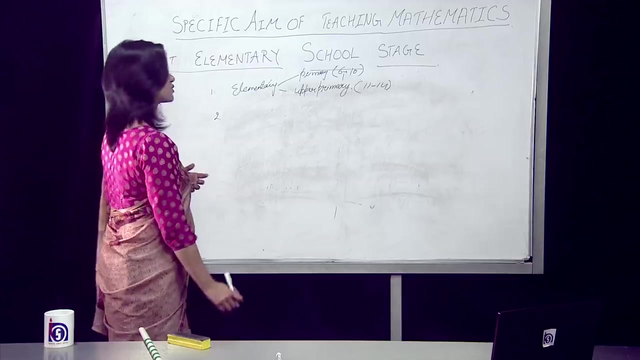 Primary education is for the children 6 to 10 years and upper primary is for the children 11 to 14 years. Elementary education is considered to be the most important level in the whole hierarchy of education. Number second. Then we learnt about the goal of mathematics education. 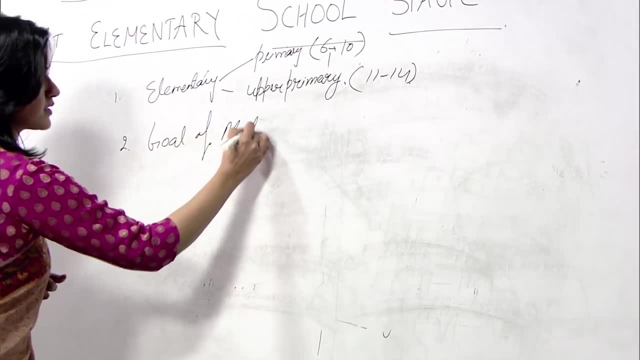 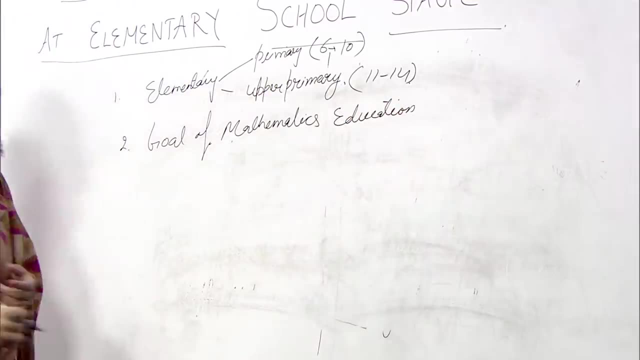 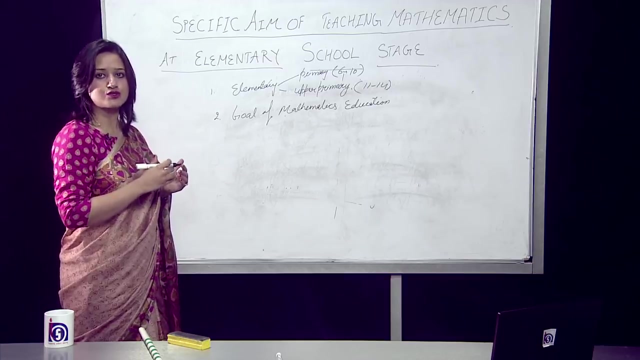 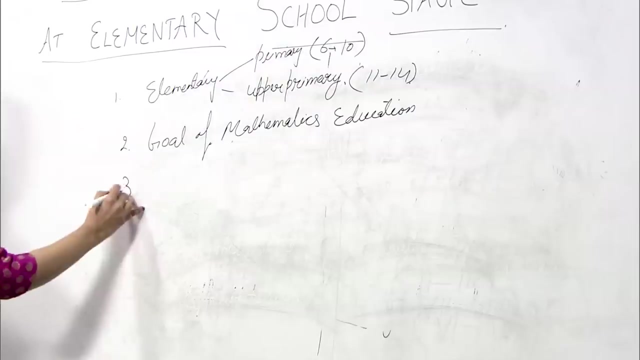 And the most important goal of mathematics education. education is to mathematize the thought process of child, So the child can apply what he has learned in the classroom and he can relate the classroom mathematics with the real life mathematics. Number third: Then we learned about specific aims, which are the instructional objectives of any topic or lesson. 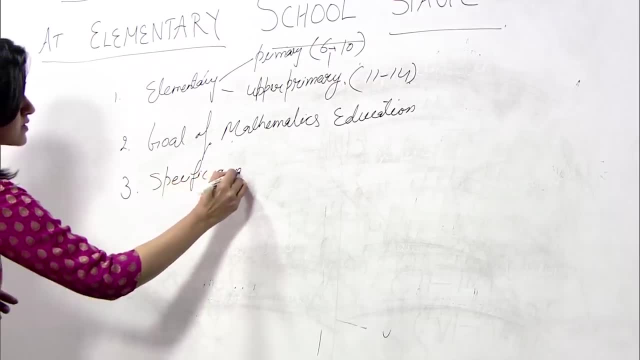 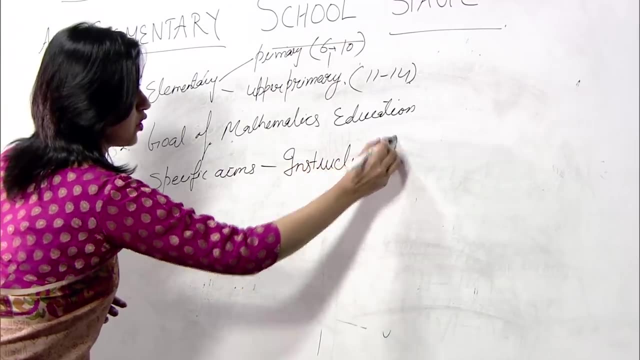 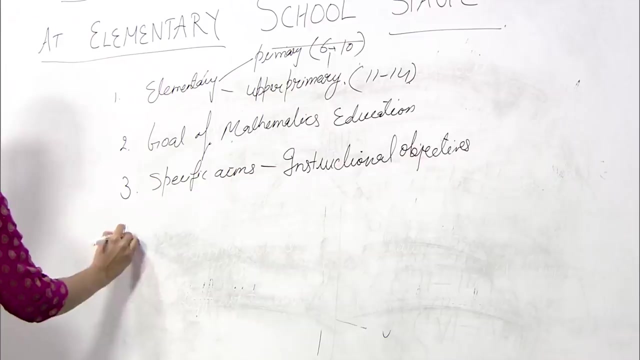 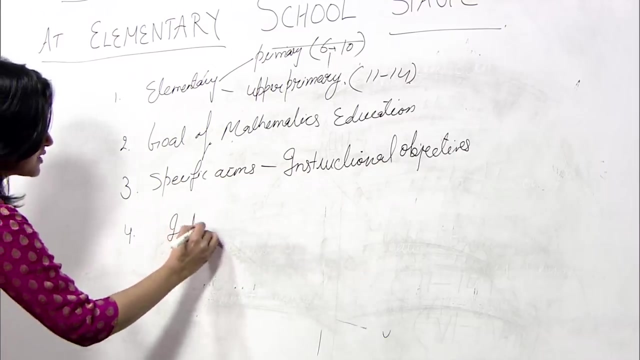 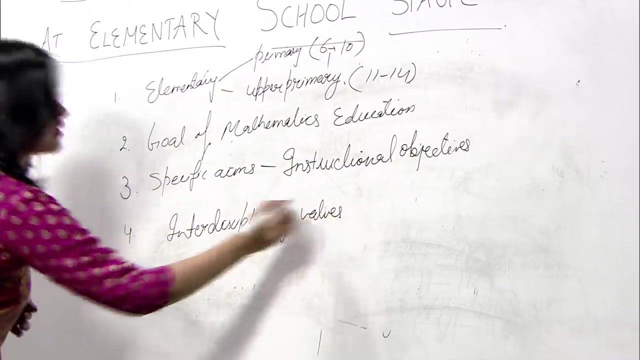 Specific aims, which are called instructional objectives. Instructional objectives. Next we did the features of specific aims of any subject or lesson. Then we learnt about the goal of mathematics education And the features of specific aims of teaching. mathematics education is to develop inter disciplinary values like critical thinking, problem solving skills, reasoning skills and 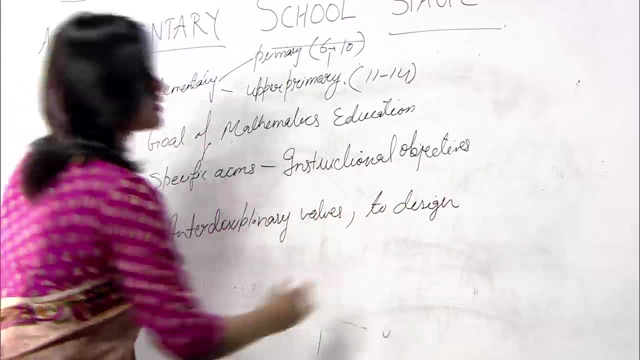 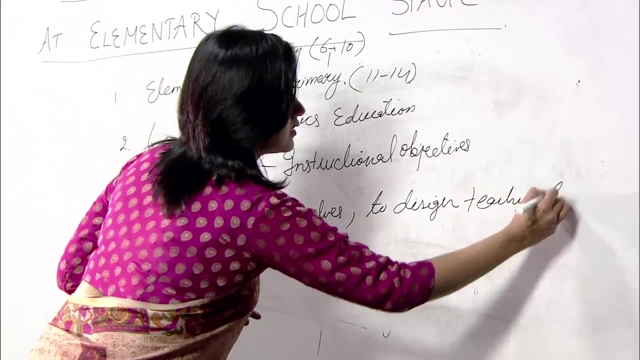 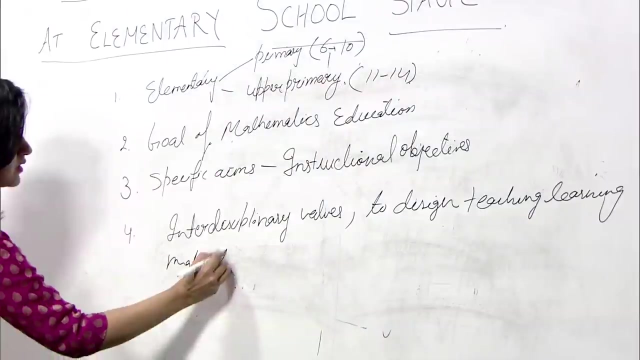 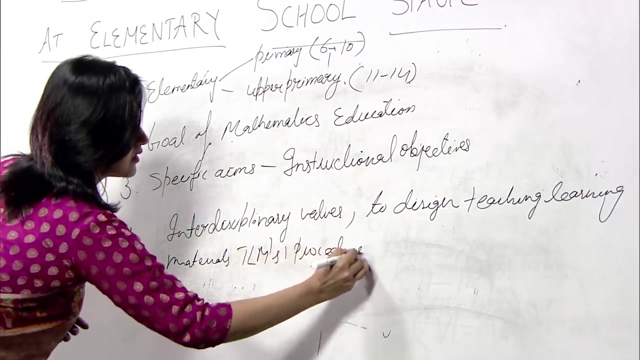 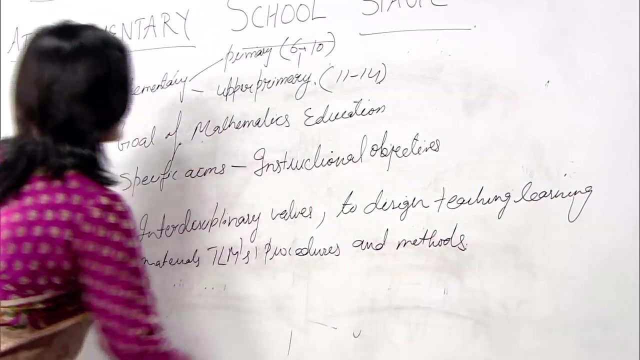 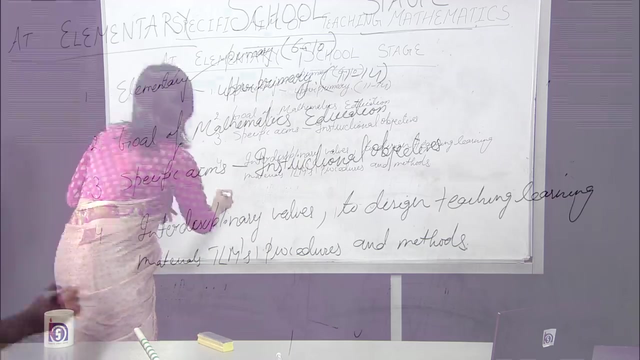 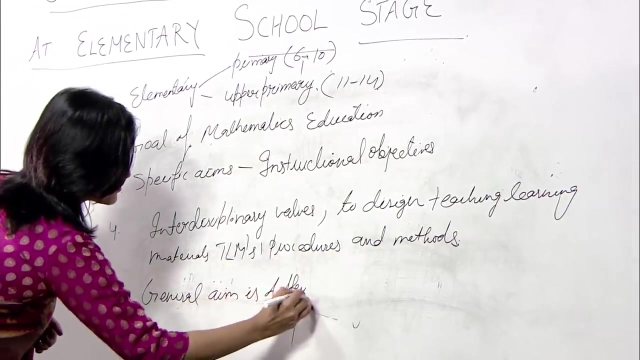 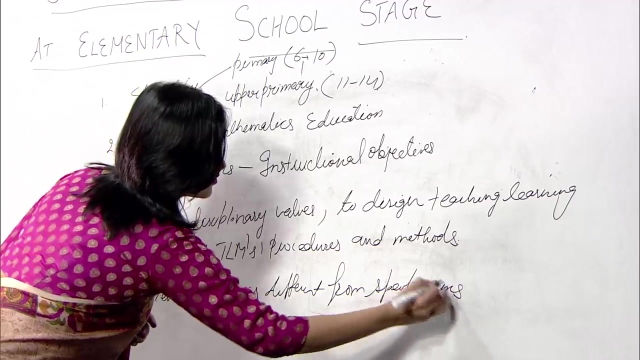 to design teaching learning materials, methods and procedures. Teaching learning materials, which we call TLMs, also procedures and methods. Then we explain the difference between general aim and the specific aim. Now general aim is different from specific aims. Specific aim, in terms that general aim, is not definite, it is not clear. they are very 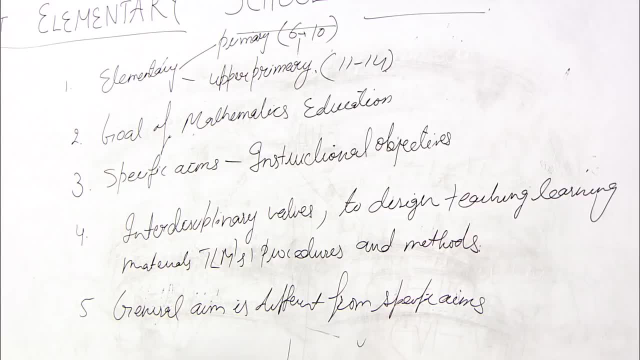 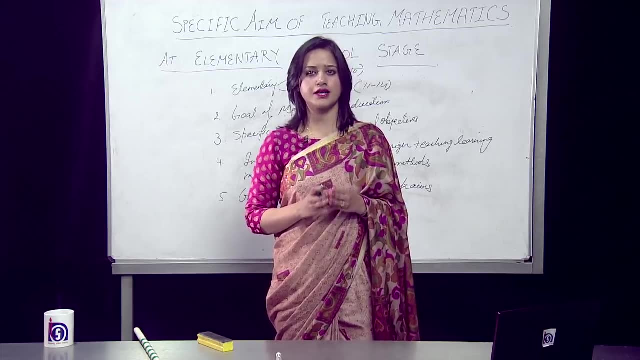 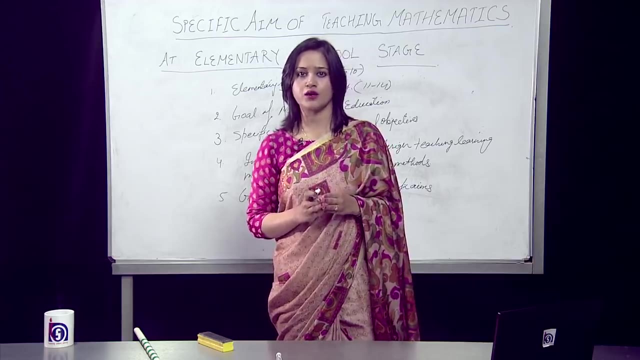 broad And they are immeasurable and they are difficult to evaluate. So this was all about the specific aims of teaching mathematics. Now, dear learners, let me give you a practice task. You can practice writing specific aims of teaching prime numbers or area of triangle. 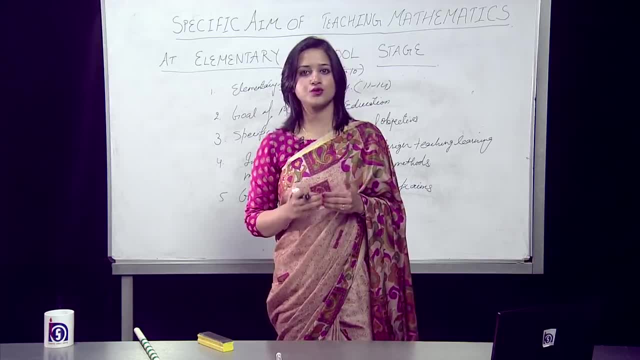 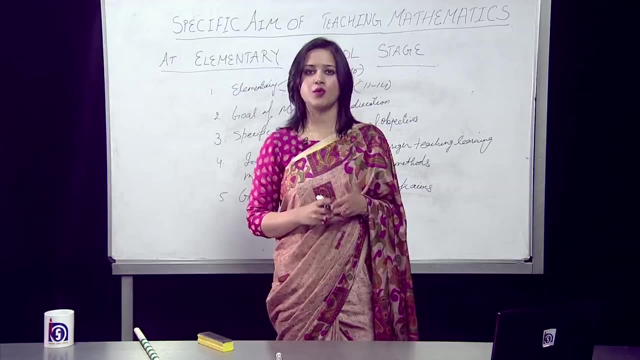 or any other topic of your choice. All you need to do is to write instructional objectives of teaching these concepts. In the words of great mathematician William Paul Thurston, mathematics is not about numbers, equations, computations or algorithms. It's about understanding.